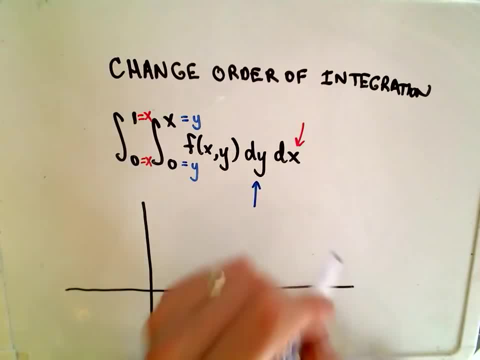 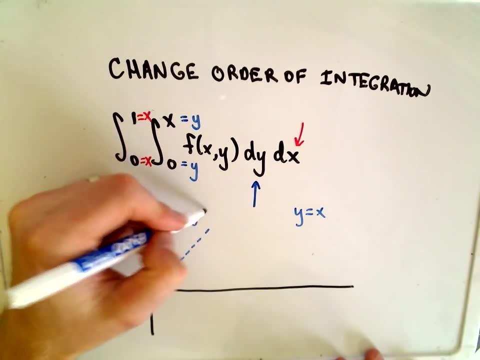 So I'm going to graph the line y equals x. Okay so y equals x, just our 45 degree line through the origin Y equals 0, which is just the x-axis. And then I'm going to do the same things. 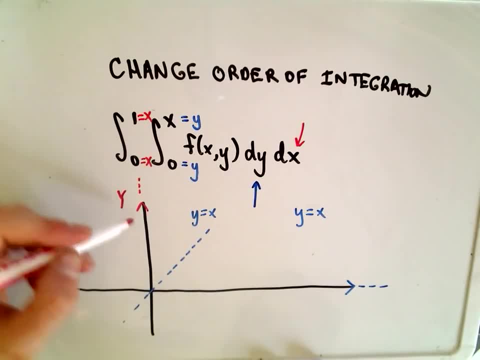 So x equals 0 would be correspondingly the y-axis, And x equals 1 will be a vertical line. Okay, so they're talking about the finite region trapped between those four curves, So to me it looks like the only region that really makes sense to be talking about would be this inside. 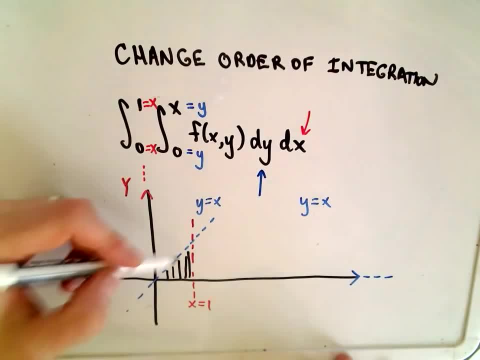 Sort of this triangular region here in the bottom right corner. Okay, so what we want to do is, again, we want to switch our limits of integration, So where we've got x first and then y, And the way I like to think about it is just to kind of in terms of the way it was originally written. 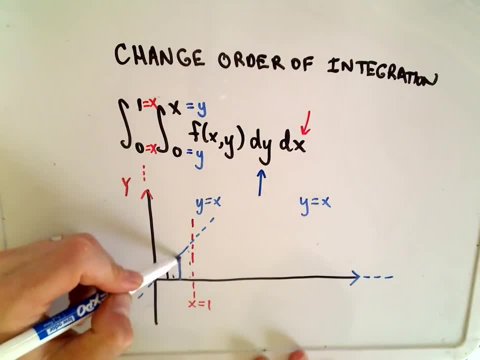 If we integrate with respect to y first, I like to think about a vertical line, Parallel, that's parallel to y, Which a vertical line would be. The bottom curve that it touches is y equals 0.. The top curve that it touches is y equals x. 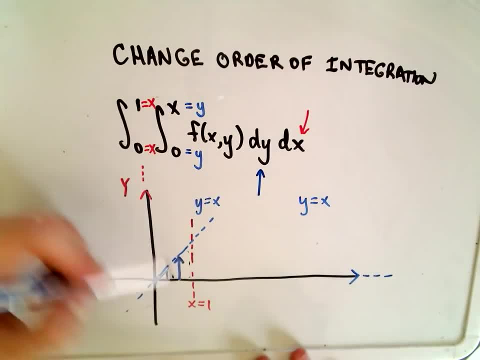 And those become our limits of integration. Likewise, if you think about the smallest x-coordinate that this region uses, it would be the x-coordinate of 0.. The largest x-coordinate that it uses would be the x-coordinate of 1.. Okay, so I'm going to try to use that same idea. 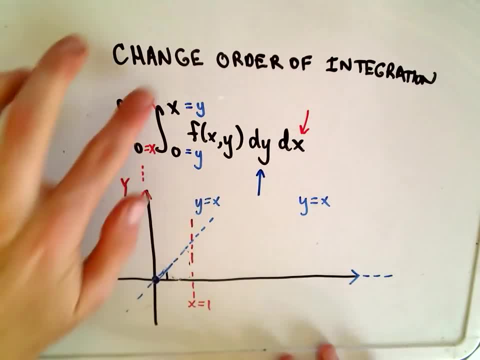 And see what happens. happens when I switch them out, Okay, so I think things might change here a little bit, so let's see what happens. So now, instead of dy dx, we want to have dx dy. Okay, so if I again we're talking about this triangular region, if I integrate, 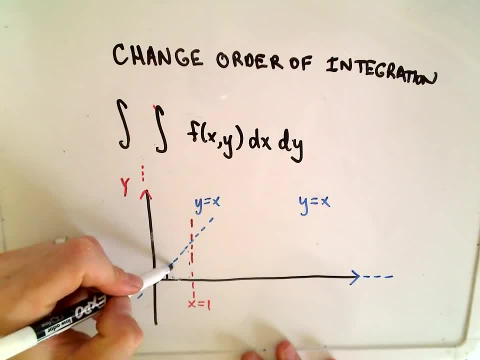 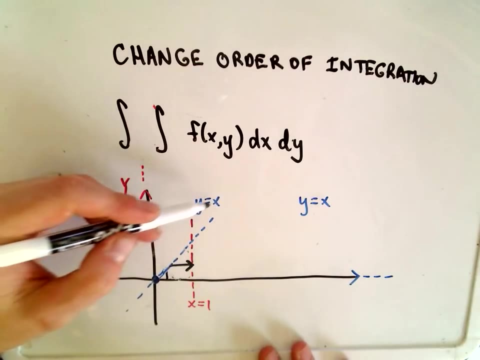 with respect to X first. now I'm going to draw a line that's parallel to the x axis, that sits inside of my region. so now notice this bottom, or the first curve. the leftmost curve that it touches is the line X equals Y, so that's going to